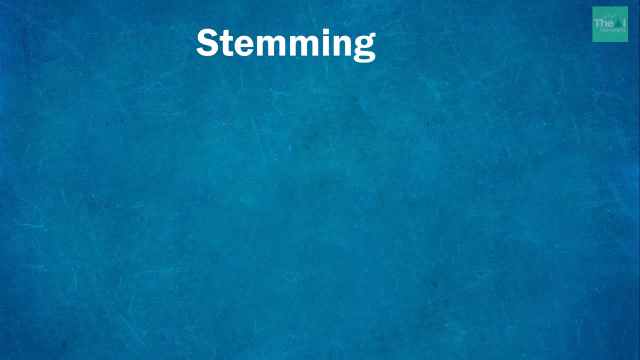 So affixes which are attached to the beginning of the word are called prefixes, For example un- in the word unknown. so the actual word is known, but if we add the un- in the beginning then it will become unknown, And the ones that are attached at the end of the word are called suffixes. 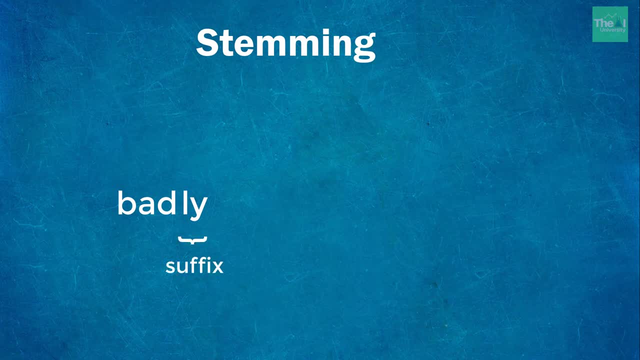 Example: ly in the word badly, so we have added ly at the end of the word bad, so it has become badly. So these are called suffixes. One thing to note here is that affixes can create or expand new form of the same word. 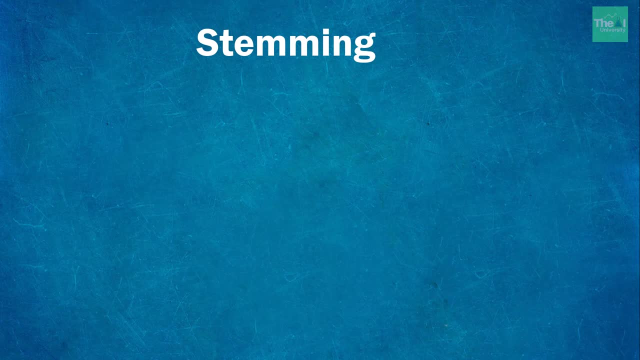 and we call it as a inflectional affixes. For example, suffix ed in the word hunted created a new form of the word hunt. On the other hand, affixes can even create new words themselves. Okay, So we call them as derivational affixes. 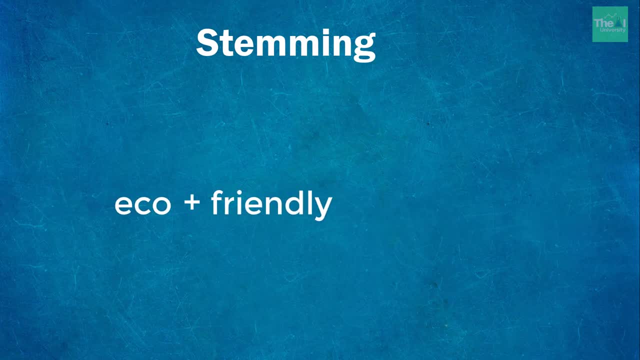 For example, prefix eco, when joined with the word friendly, creates altogether a new word called eco-friendly. Okay, So these are called derivational affixes. So we use stemming to chop off these affixes to bring the word into its root form, or reducing. 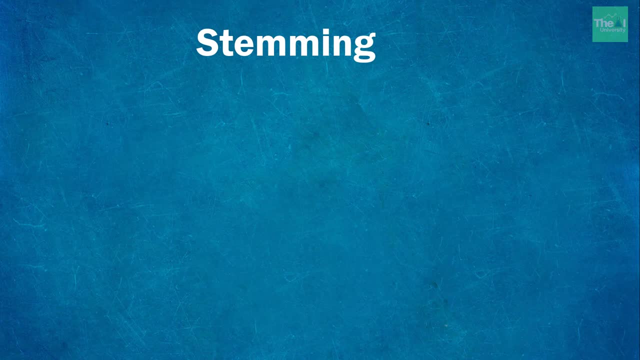 word to their word stems. One of the advantages of stemming process is that it can be used to correct spelling errors from the tokens. Stemmers are simple to use and run very fast, And if, in case, speed and performance are important aspects in your NLP model, then stemming is. 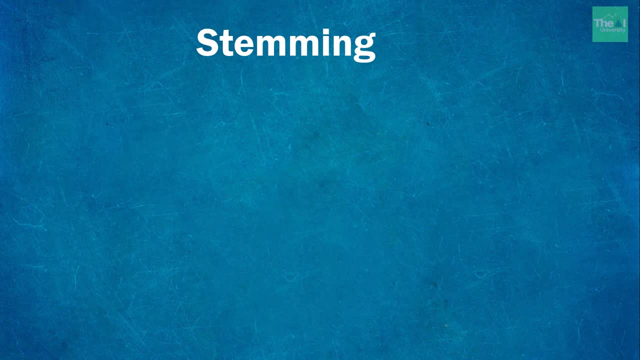 certainly your best choice. There is one more process called lemmatization, Which is used to reduce word to its base form and grouping together different forms of the same word. I will be covering this topic in the next video, as well as difference between stemming. 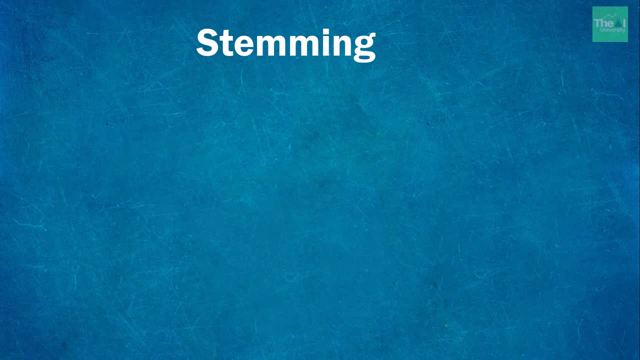 and lemmatization. Both stemming and lemmatization are widely used in indexing SEOs, ie search engine optimizations, web search results, etc. That's it. We want to search a word called care On google. the search will look for caring and cares, as care is the stem of the word. 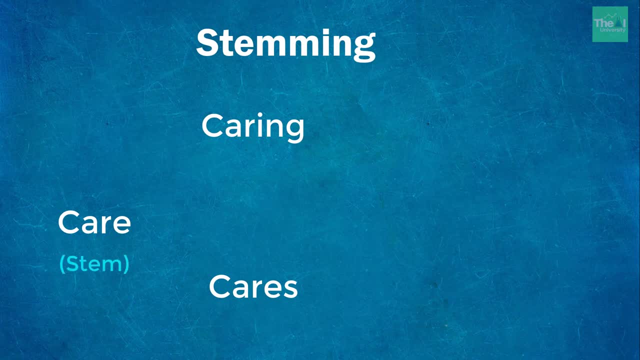 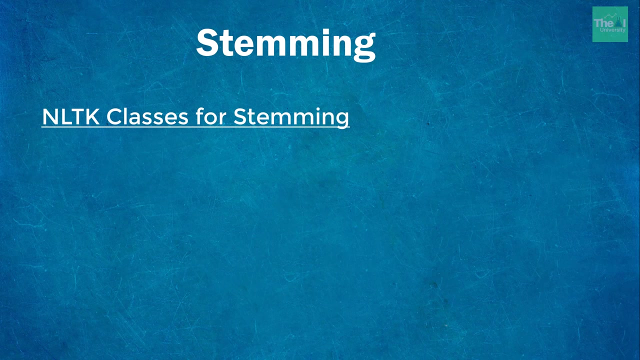 of both of these words. So care is the stem of both caring as well as cares. So in NLTK, stemmers are available in different languages, and in English we normally use either Porter Stemmer or Lancaster Stemmer. Ok, Here I will use Porter Stemmer throughout, because it is considered as most optimized. 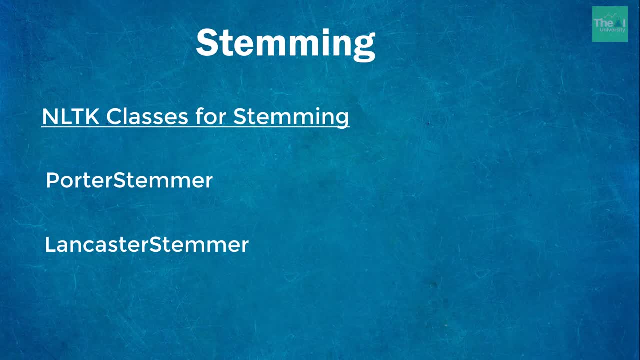 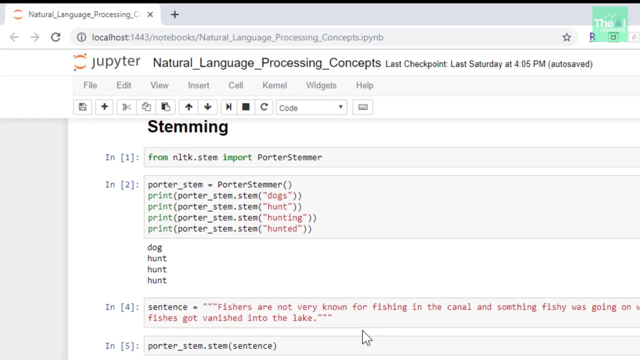 with respect to its speed. So let's move on to the Python code associated with stemming. Let me open my Jupyter notebook real quick here. Ok, and here is the stemming. Ok, I will start with the, you know, stemming the individual words first. 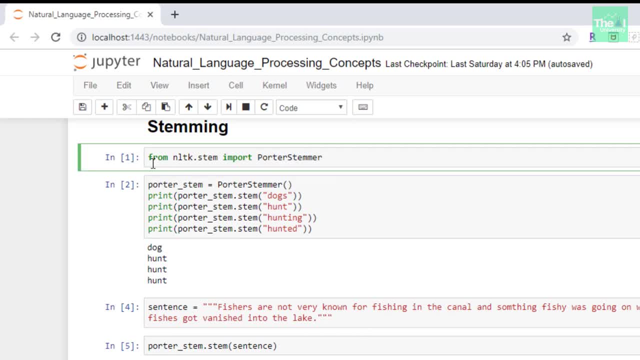 So in the first cell, as you can see here, NLTK dot stem package, which is this one, contains several stemming classes. Porter Stemmer is the one of those classes which I am importing here. Ok, And in the next cell I am creating the object of Porter Stemmer here. 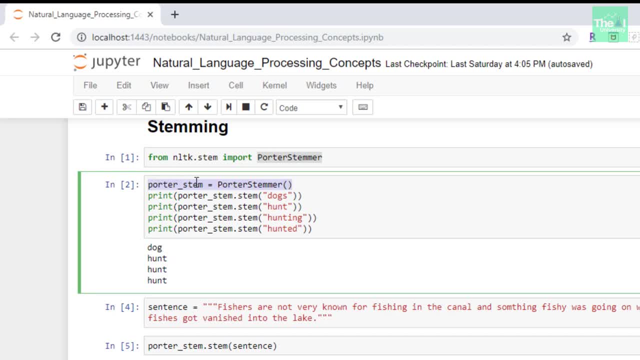 Ok, Ok, Ok. And I have created this object of Porter Stemmer and in the next, you know, after creating this Porter Stemmer object, I try to generate the stem words for the word dogs: ok, hunt, hunting and hunted, Ok, Notice, Now Porter Stemmer is giving the root word- ok, root stem of the word dogs by simply removing 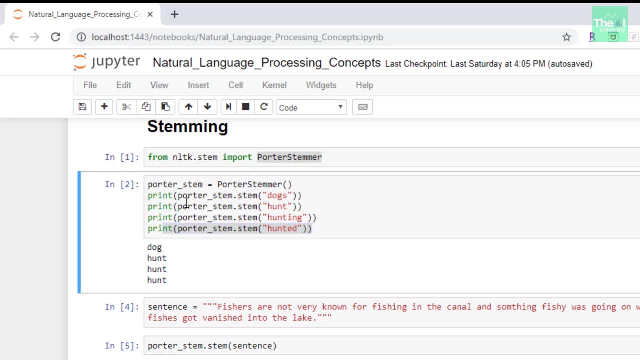 s. So this Porter Stemmer basically removed the s and generated the root word dog ok by simply removing s. But if you look at this- hunt ok, Hunt hunting and hunted Ok, They are actually stemmed to the same word called hunt ok, which is a root word. 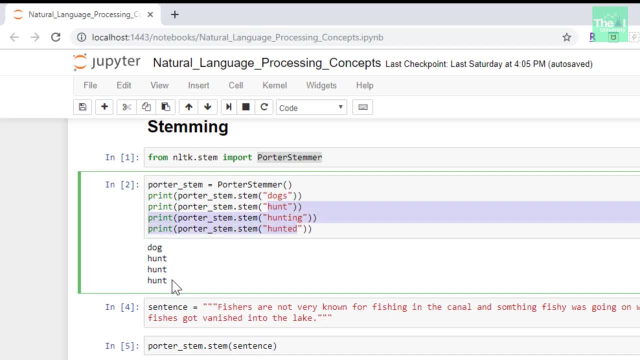 So all of these three words were stemmed to a single root word: hunt. ok, Alright, so that's what I wanted to show you: how can we stem the individual words here, ok, and what output actually we would get when we stem The same form of an individual word, which we did here: hunt. we used hunt different forms. 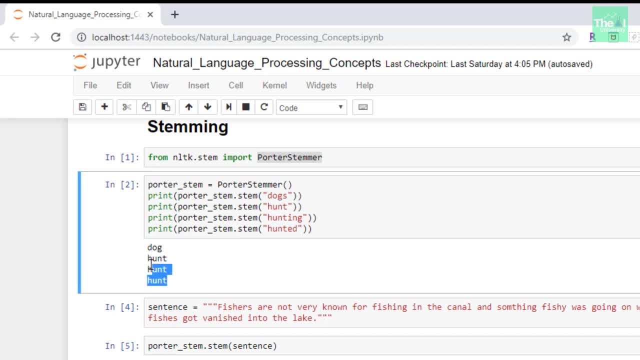 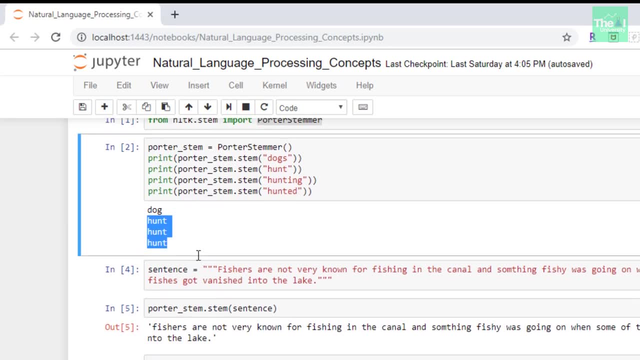 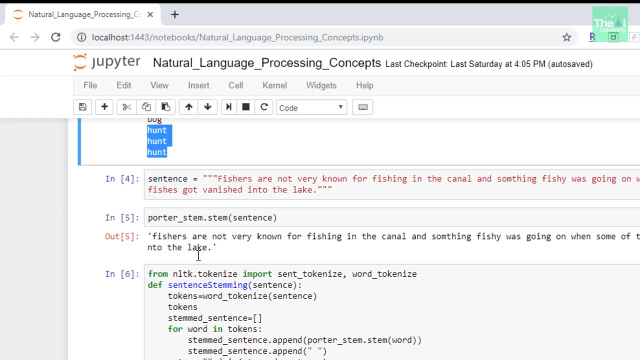 of word hunt here and actually stemmed it to single word hunt. Now let's see how can we stem a sentence now. ok, So let me scroll up a bit and let's say we have this sentence which says: fishers are not very known for fishing in the canals. 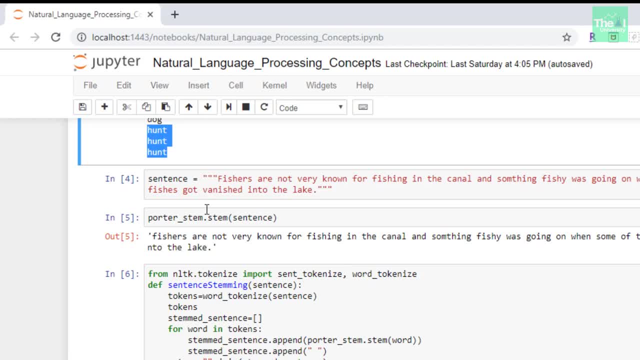 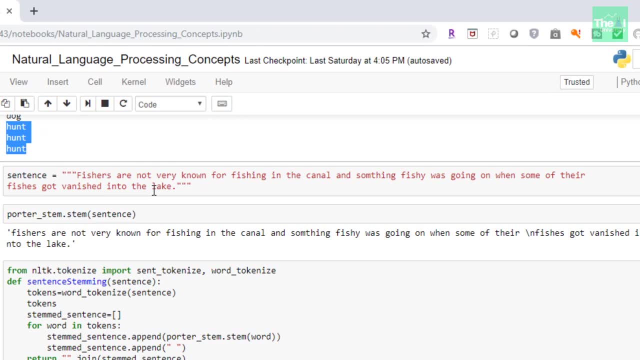 Ok, They were fishing in the canal and something fishy was going on when some of their fishes got vanished into the lake. ok, Now let's stem this sentence using Porter underscore: stem dot, stem. ok, by passing this sentence as an argument here. So I am passing this particular sentence as an argument here into the Porter underscore. 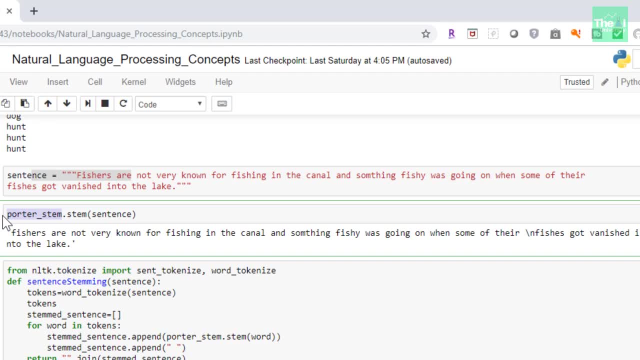 stem dot stem. And remember this: Porter underscore stem. Porter underscore stem is an object of Porter stemmer. ok, So when we lineup this, we can see that there was no change in the sentence. If you see the sentence as well as this, if you compare these two, 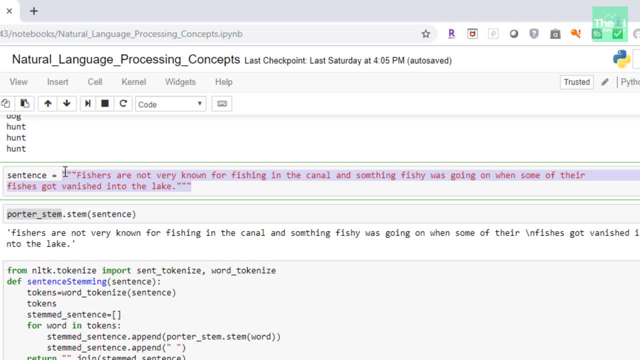 There was no change at all in the sentence after performing stemming. The reason is that the stemmer sees the entire word sentence as a word, So this stem: use this entire sentence. It at a sentence as a word. Ok, So very nice. this is the sentence. Energy source sense wasting all the important things. Bear in mind that就是 in the context, because in the context, if I call this language here, We can see exactly what we are doing here- is that when am commonly think about ur r mera, leitbo multiple. 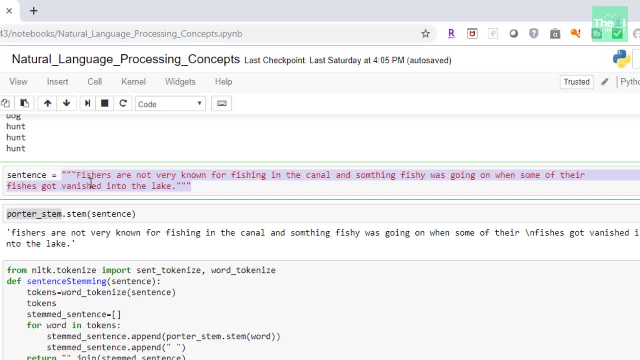 word. okay, and that's the reason it will return the sentence as it is. the solution, therefore, is to stem each word in the sentence and return it as a combined sentence. okay, and in order to separate the sentence into words, we can use tokenizer, which I am using here. you can see, and if you don't know about 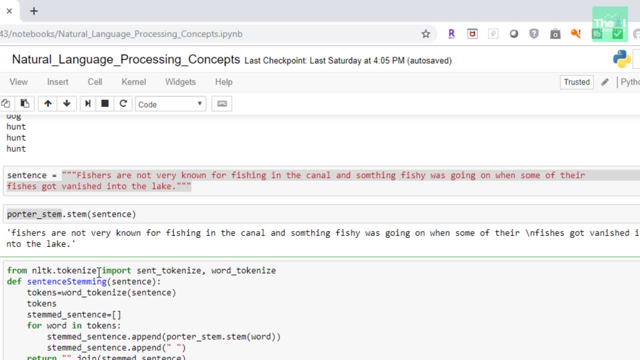 tokenization step. then you can very well watch a separate video which I have created on tokenization. I will give the link of it in the I button above. okay, so to separate the sentence into words, we can use tokenizer. okay, and I have used this and nltktokenize package and more specifically, the 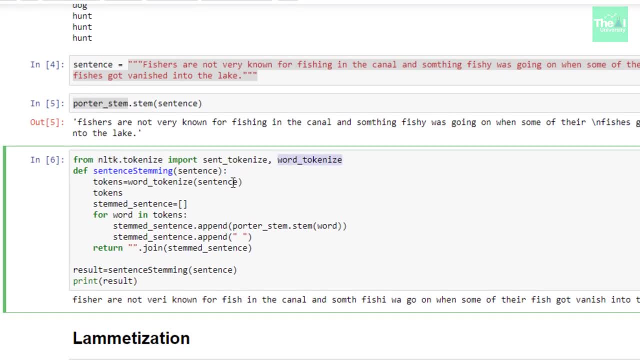 word tokenizer. we can use it for specific reasons also. you can use tokenizer in the tokenization step. then you can very well watch a separate video which I have world underscore, tokenize class of it- okay, and I'm using it here in this particular function. okay. so using NLTK tokenizer, we can separate a sentence into words and inside this you can see. 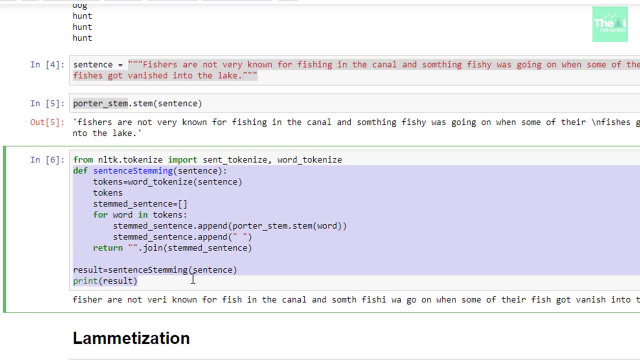 I have created this function. so, inside this function, I first received this complete sentence as an argument here- okay, and then I performed word tokenization on entire sentence here- okay. so I created separate tokens- word tokens- from this sentence- okay, all right, and the result of this is then stored in a variable called tokens. okay, then what I did was I initialized. 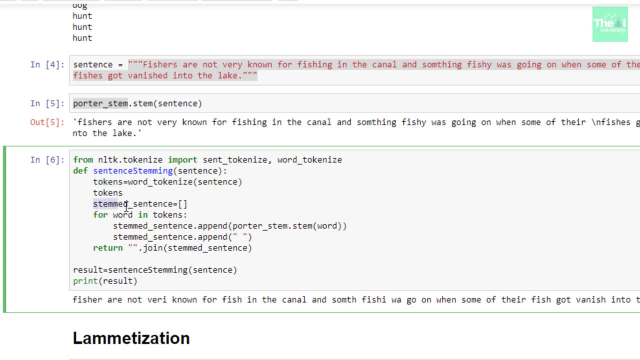 an empty list called a stemmed sentence. okay, so I created this empty list and after this, I used a for loop to iterate over each word in the sentence in order to stem them, using potter underscore: stemmer, dot, stem okay, and appending that a stemmed word into this.